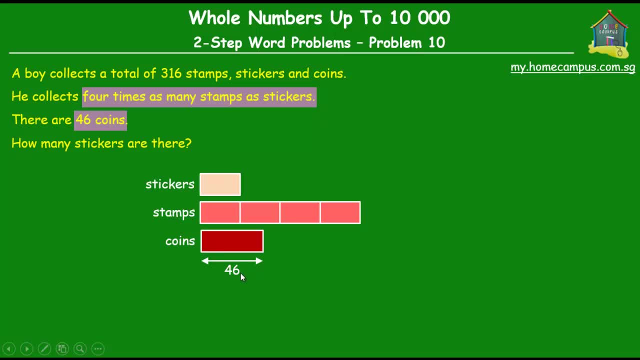 we put a unit for the coins and that's equal to 46.. Now the last thing we know is there are a total of 316 stamps, stickers and coins. So all of these units over here together they are equal to 316.. So on the model, we mark that as well. All right now, from here what we have to find out. 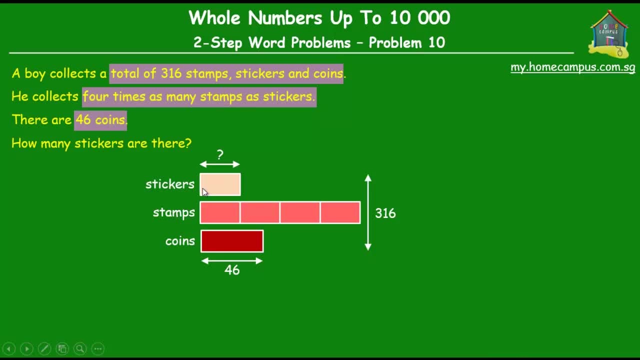 is how many stickers are there. So what we have to find out is what this little unit over here is equal to, and that's the number of stamps. So let's find out how many stickers are there. All right now. what do we see from the model diagram over here? What we see is that if we 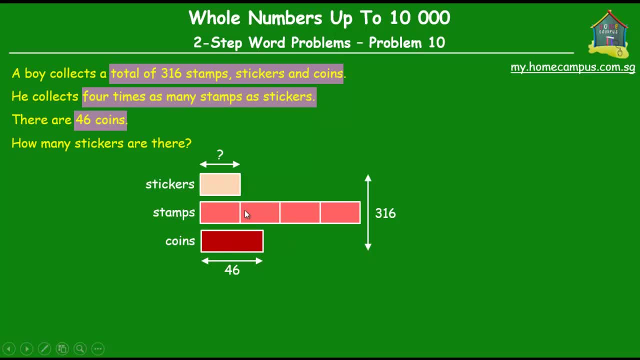 remove the number of coins from the total number of stickers, stamps and coins, which is 316, then what we will have left is just the stickers and the stamps, And we know that together, the stickers and the stamps are five equal units. So that will take us to the final answer. All right, 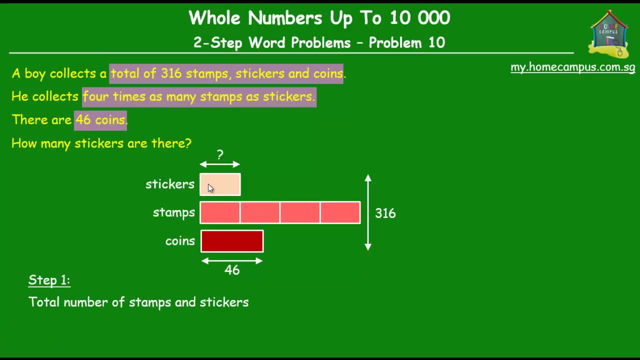 we'll solve that one step at a time. So, first of all, what we will do is we'll find out the total number of coins from the total number, which is 316.. So we do 316 minus 46.. And on the right of 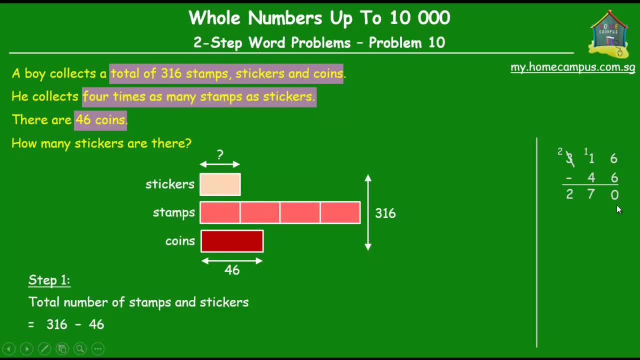 the screen we do the subtraction. the detailed steps I'm not going to go through because we've already covered that in several other tutorials on subtraction. So 316 minus 46 is equal to 270.. Now on the model diagram, we remove that and this is what 270 stands. 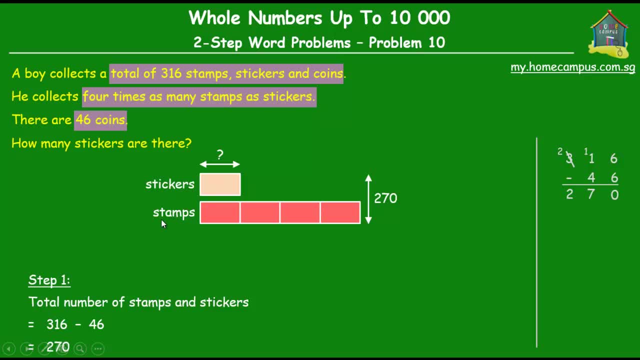 It stands for the total number of stickers and stamps. Now, from the model it's again quite clear that these units over here for the stickers and the stamps are equal in size And there are altogether five units, one for stickers and four for stamps, and they are 270 in number. 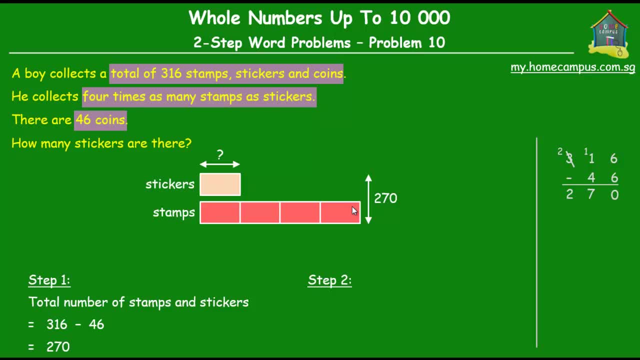 So all we have to do now to find out the number of stickers is to divide 270 by the five units. So we do 316 minus 46.. And on the right of the screen we do 316 minus 46. And on the left of 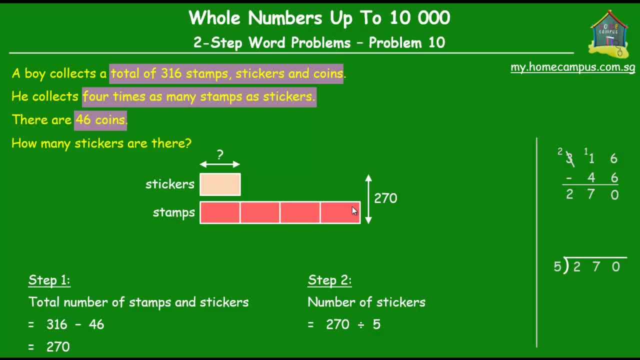 the screen we do 270 divided by five, And on the right of the screen we do the working. So five goes into 27 five times, and five times five is 25, we are left with two and we bring down the.